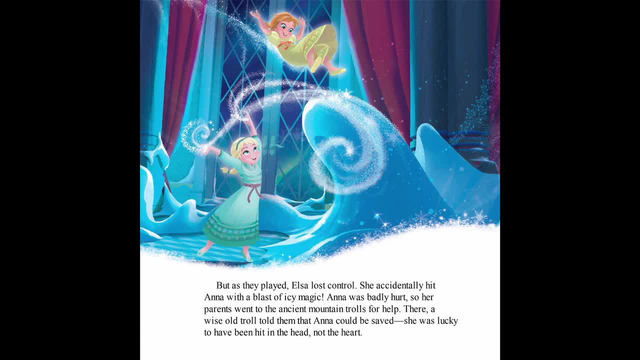 But as they played, Elsa lost control. She accidentally hit Anna with a blast of icy magic. Anna was blown away. She was badly hurt. So her parents went to the ancient mountain trolls for help. There a wise old troll told them that Anna could be saved. She was lucky to have been hit in. 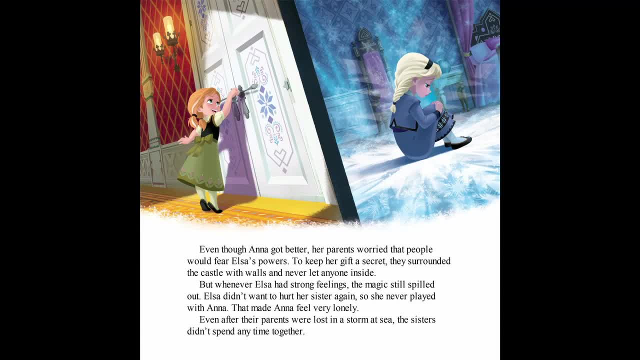 the head, not the heart. Even though Anna got better, her parents worried that people would fear Elsa's powers To keep her gift a secret. they surrounded the castle with walls and never let anyone inside. But whenever Elsa had strong feelings, the magic still. 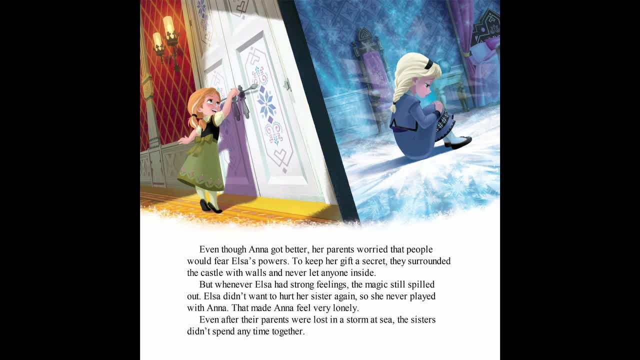 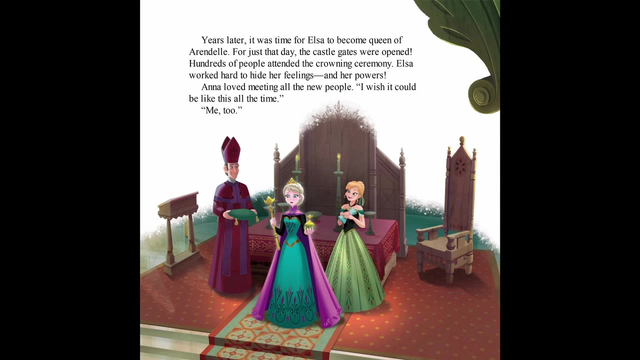 spilled out. Elsa didn't want to hurt her sister again, so she never played with Anna. That made Anna feel very lonely. Even after their parents were lost in a storm at sea, the sisters didn't spend any time together. Years later, it was time for Elsa to become Queen of Arendelle. For just that day, the 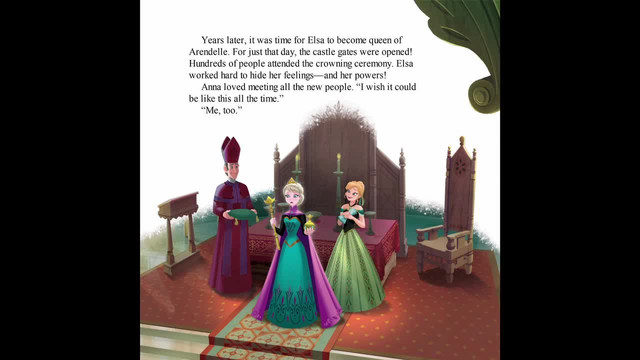 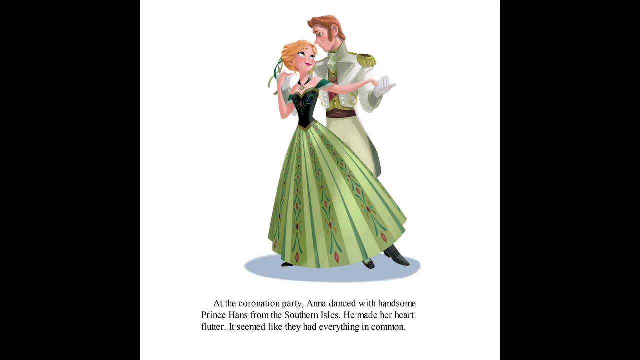 castle gates were opened. Hundreds of people attended the crowning ceremony. Elsa worked hard to hide her feelings and her powers. Anna loved meeting all the new people. I wish it could be like this all the time, Me too. At the coronation party, Anna danced with handsome Prince Hans from the Southern Isles. 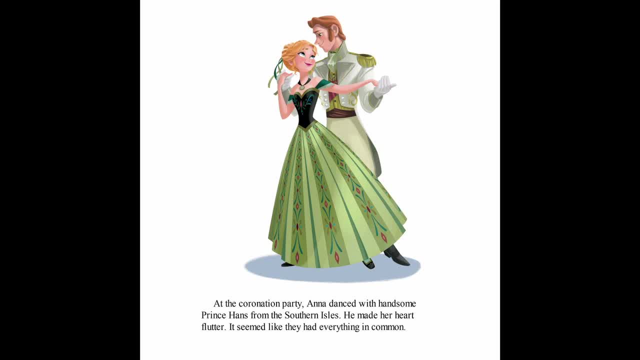 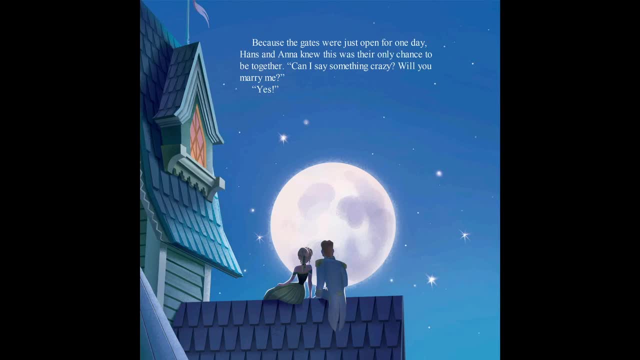 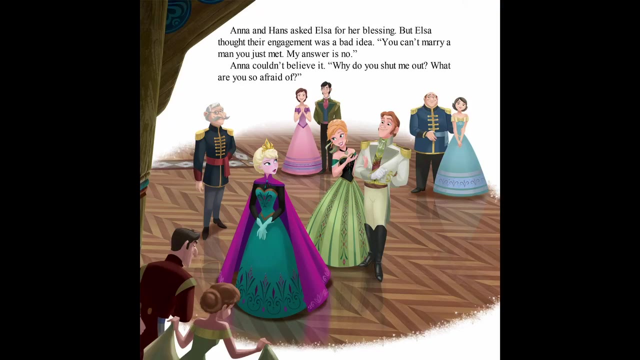 He made her heart flutter. It seemed like they had everything in common, Because the gates were just open for one day. Hans and Anna knew this was their only chance to be together. Can I say something crazy? Will you marry me? Yes, 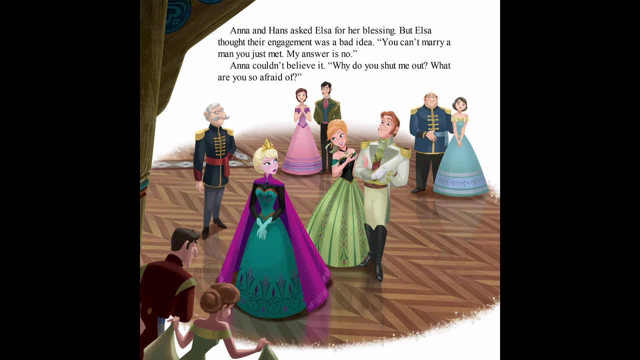 Anna and Hans asked Elsa for her blessing, But Elsa thought their engagement was a bad idea. You can't marry a man you just met. My answer is no. Anna couldn't believe it. Why do you shut me out? What are you so afraid of? 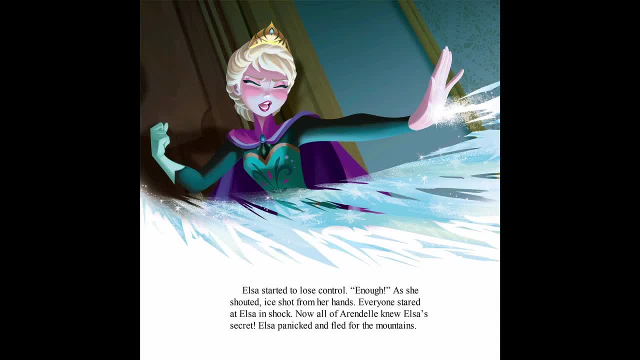 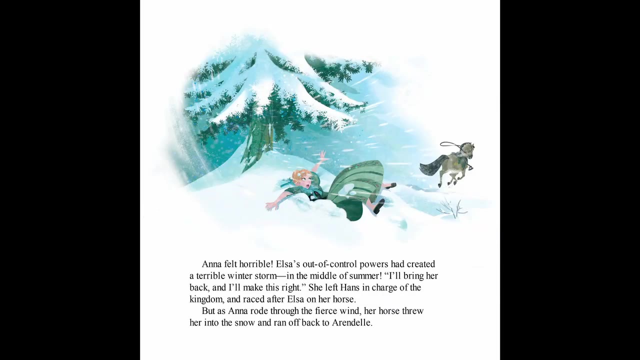 Elsa started to lose control Enough As she shouted: ice shot from her hands. Oh no, Everyone stared at Elsa in shock. Now all of Arendelle knew Elsa's secret. Elsa panicked and fled for the mountains. Anna felt horrible. Elsa's out-of-control powers had created a terrible winter storm. 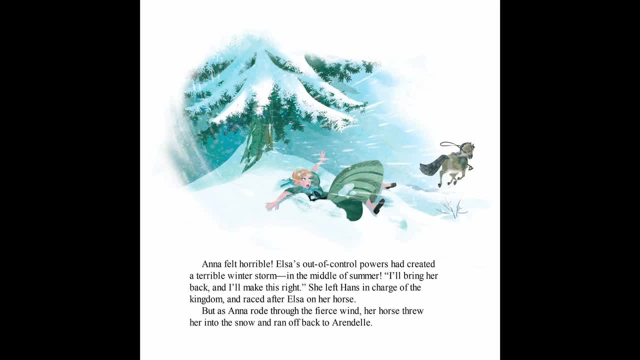 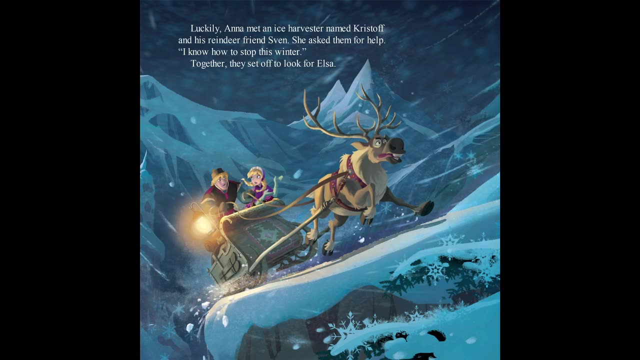 in the middle of summer. I'll bring her back and I'll make this right. She left Hans in charge of the kingdom and raced after Elsa on her horse, But as Anna rode through the fierce wind, Her horse threw her into the snow and ran off back to Arendelle. Luckily, Anna met an 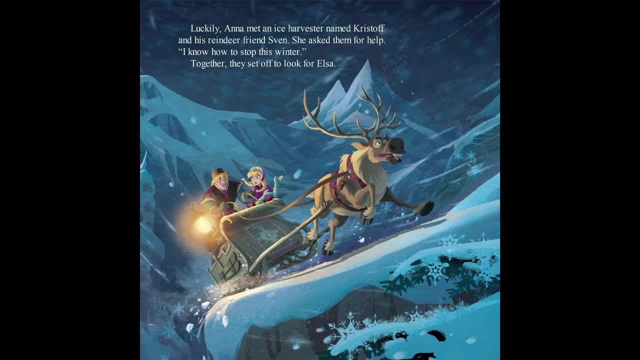 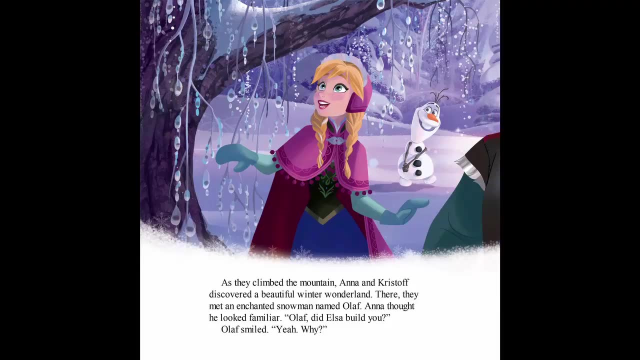 ice harvester named Kristoff and his reindeer friend Sven. She asked them for help. I know how to stop this winter. Together, they set off to look for Elsa. As they climbed the mountain, Anna and Kristoff discovered a beautiful winter wonderland. 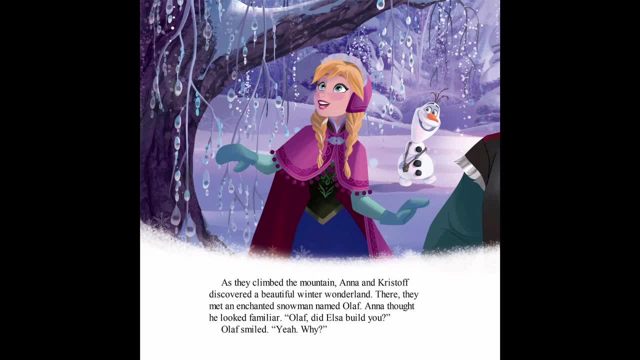 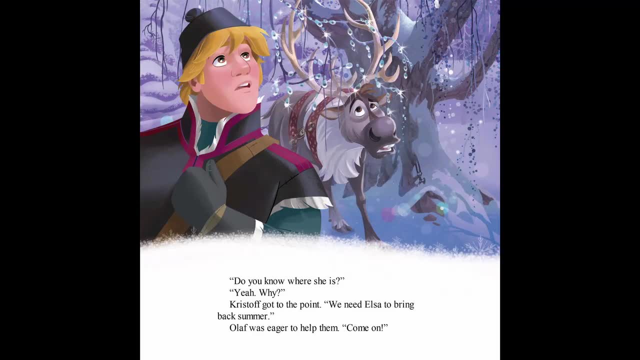 There they met an enchanted snowman named Olaf. Anna thought he looked familiar. Olaf, did Elsa build you? Olaf smiled: Yeah, why Do you know where she is? Yeah, why Kristoff got to the point. We need Elsa to bring back summer. 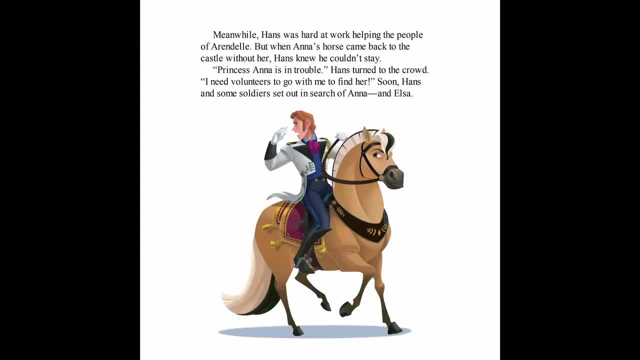 Olaf was eager to help them Come on. Meanwhile Hans was hard at work helping the people of Arendelle. But when Anna's horse came back to the castle without him, Hans knew he couldn't stay. Princess Anna is in trouble. 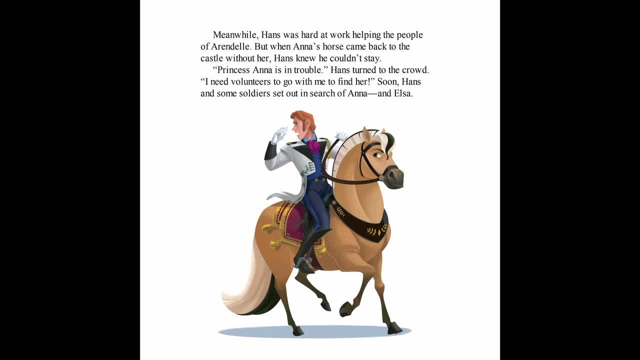 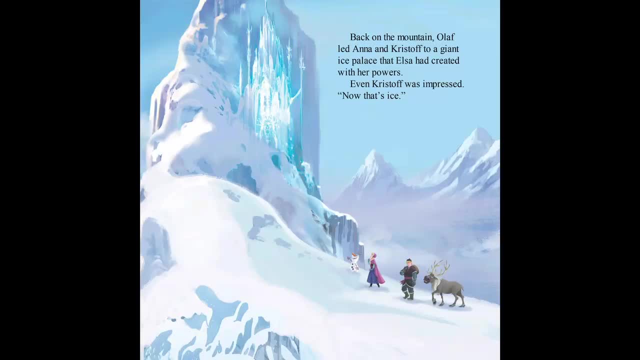 Hans turned to the crowd. I need volunteers to go with me to find her Soon. Hans and some soldiers set out in search of Anna and Elsa. Back on the mountain, Olaf led Anna and Kristoff to a giant ice palace that Elsa had created. 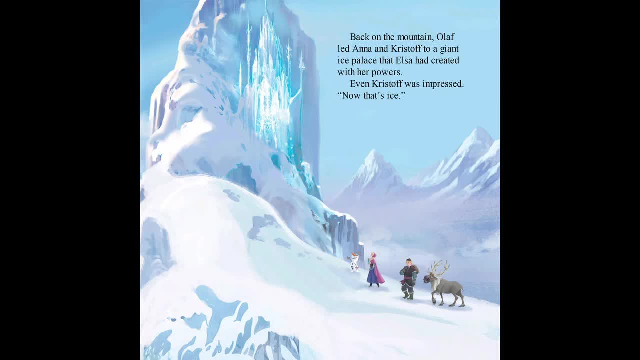 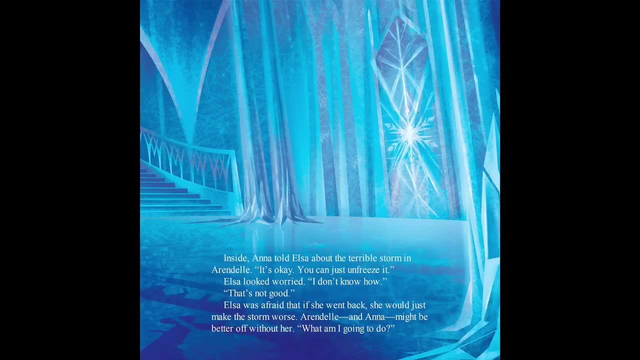 with her powers. Even Kristoff was impressed. Now that's ice. Elsa's Ice Palace Inside. Anna told Elsa about the giant ice palace Inside. Anna told Elsa about the terrible storm in Arendelle. It's okay, You can just unfreeze it. 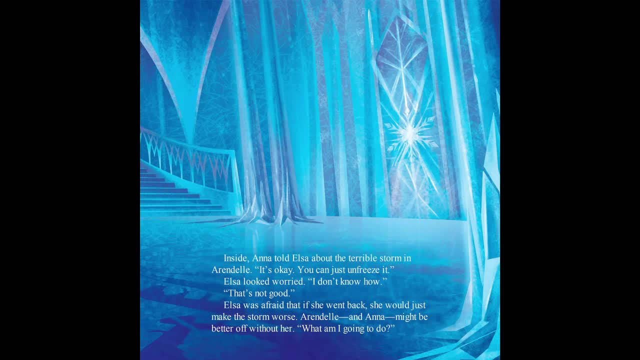 Elsa looked worried. I don't know how. That's not good. Elsa was afraid that if she went back she would just make the storm worse. Arendelle and Anna might be better off without her. What am I going to do? 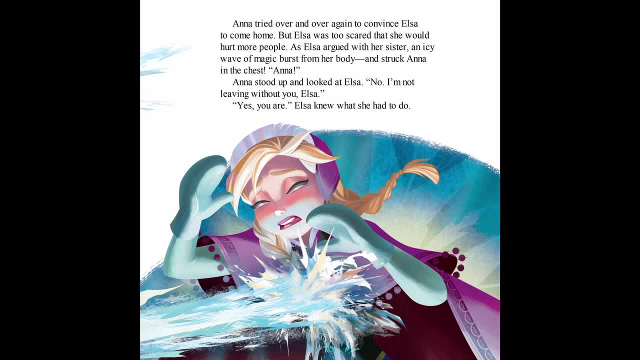 Anna tried over and over again to convince Elsa to come home, but Elsa was too scared that she would hurt more people. As Elsa argued with her sister, an icy wave of magic burst from her body and struck Anna in the chest. Anna, Anna stood up and looked at Elsa. 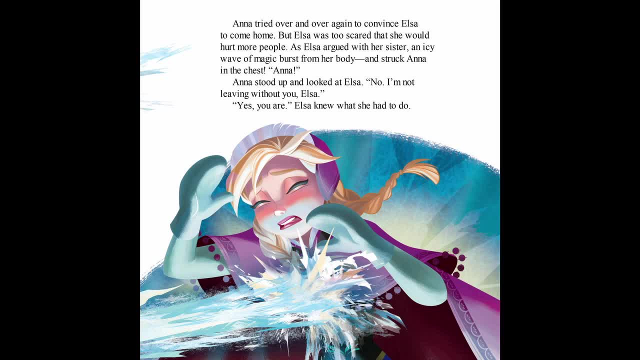 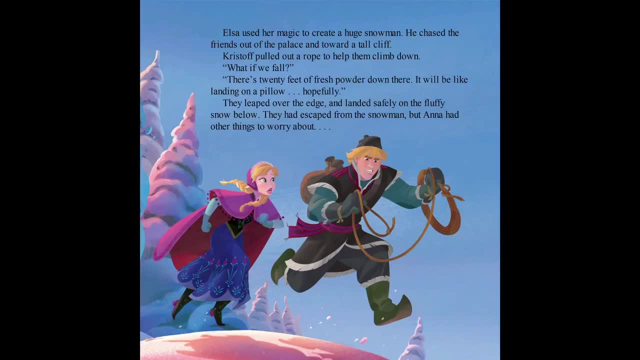 No, I'm not leaving without you. Elsa- Yes, you are. Elsa knew what she had to do. Elsa used her magic to create a huge snowman. He chased the friends out of the palace and toward a tall cliff. Kristoff pulled out a rope to help them climb down. 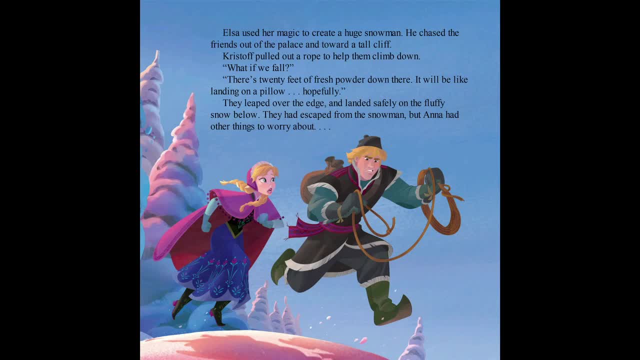 What if we fall? There's 20 feet of fresh powder down there. It'll be like landing on a pillow. Hopefully They leaped over the edge and landed safely on the fluffy snow below. They had escaped from the snowman, but Anna had other things to worry about. 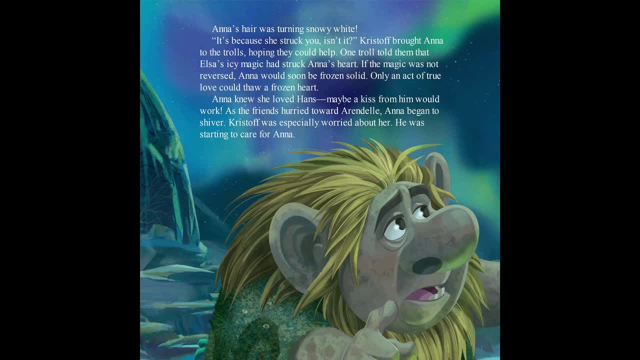 Anna's hair was turning snowy white. It's because she struck you, isn't it? Kristoff brought Anna to the trolls, hoping they could help. One troll told them that Elsa's icy magic had struck Anna's heart. If the magic was not reversed, Anna would soon be frozen solid. 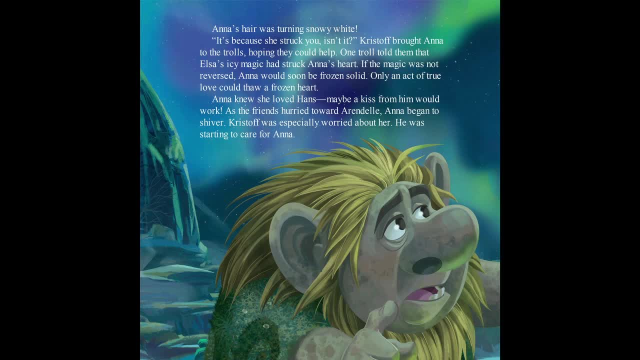 Only an act of true love could thaw a frozen heart. Anna knew she loved Hans. Maybe a kiss from him would work. As the friends hurried toward Arendelle, Anna began to shiver. Kristoff was especially worried about her. He was starting to care for Anna. 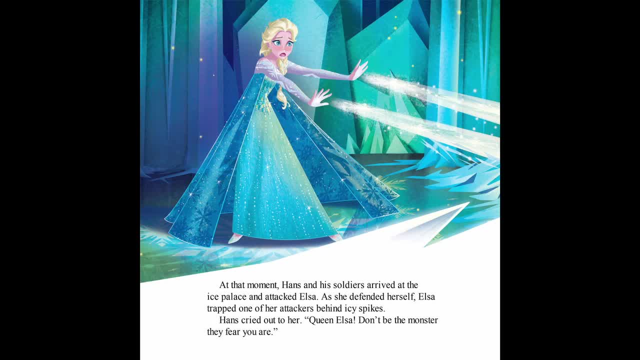 At that moment, Hans and his soldiers arrived at the Ice Palace and attacked Elsa As she defended herself. Elsa trapped one of her attackers behind icy spikes. Hans cried out to her Queen: Elsa, Don't be the monster they fear you are. 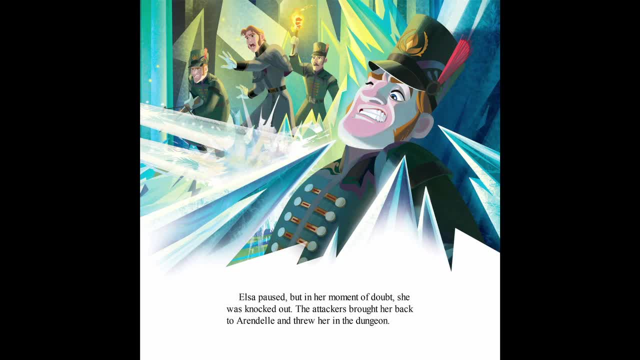 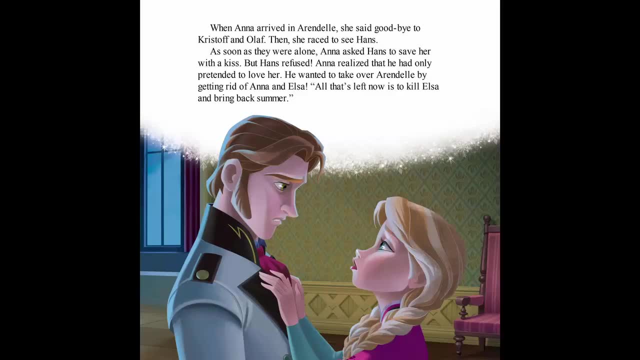 Elsa paused, but in her moment of doubt she was knocked out. The attackers brought her back to Arendelle and threw her in the dungeon. When Anna arrived in Arendelle she said goodbye to Kristoff and Olaf. Then she raced to see Hans. 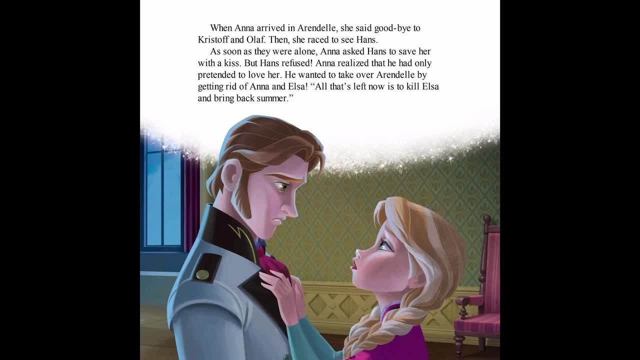 As soon as they were alone, Anna asked Hans to save her with a kiss, But Hans refused. Anna realized that he had only pretended to love her. He wanted to take over Arendelle by getting rid of Anna. He wanted to save Anna and Elsa. 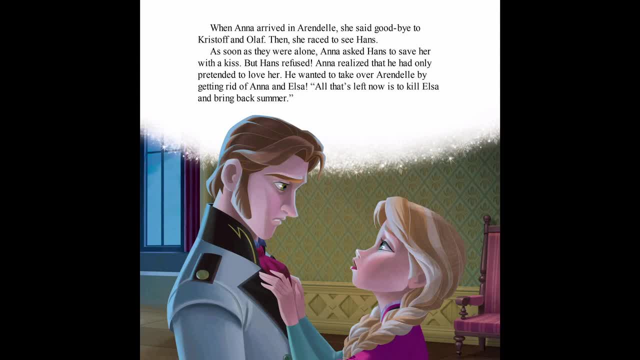 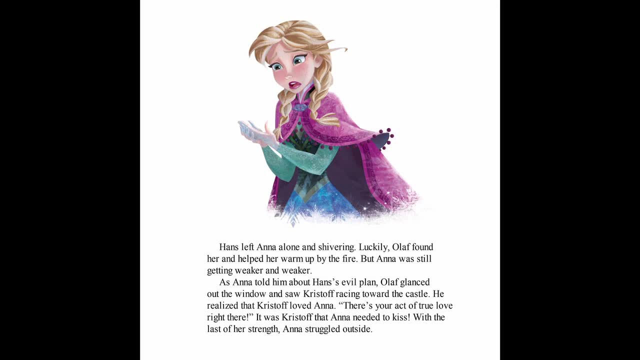 All that's left now is to kill Elsa and bring back Summer. Hans left Anna alone and shivering. Luckily, Olaf found her and helped her warm up by the fire, But Anna was still getting weaker and weaker As Anna told him about Hans' evil plan. 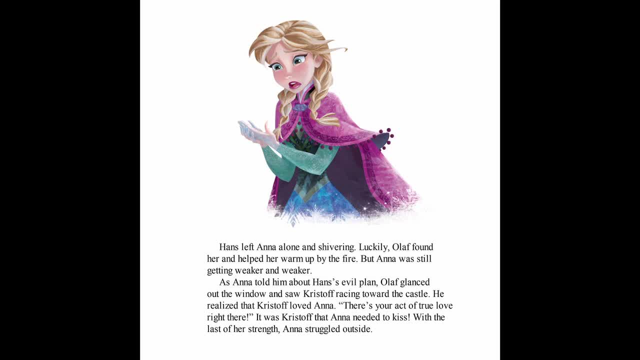 Olaf glanced out the window and saw Kristoff racing toward the castle. He realized that Kristoff loved Anna. There's your act of true love right there. It was Kristoff that Anna needed to kiss. With the last of her strength, Anna struggled outside. 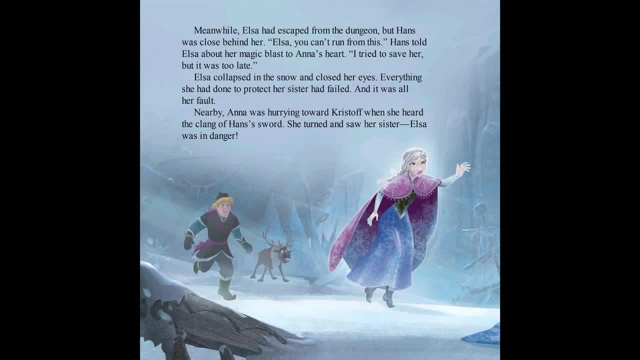 Meanwhile, Elsa had escaped from the dungeon, but Hans was close behind her. Elsa, You can't run from this. Hans told Elsa about her magic blast to Anna's heart. I tried to save her, but it was too late. Elsa collapsed in the snow and closed her eyes. 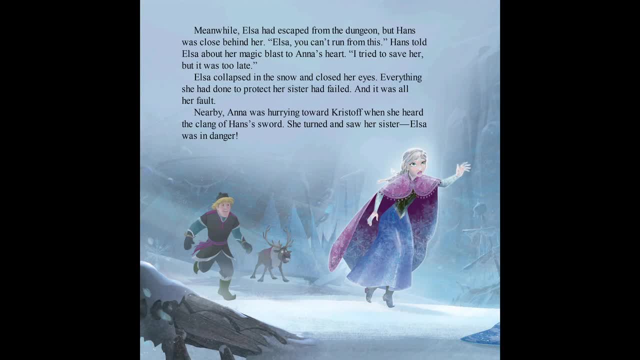 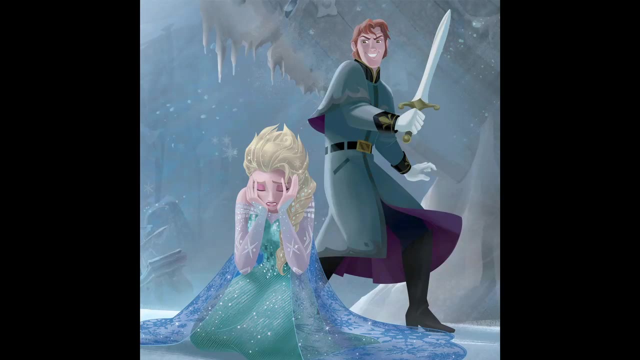 Everything she had done to protect her sister had failed, And it was all her fault. Nearby Anna was hurrying toward Kristoff. when she heard the clang of Hans' sword, She turned and saw her sister, Elsa, was in danger. Instead of saving herself and running to Kristoff, Anna leaped in front of her sister. 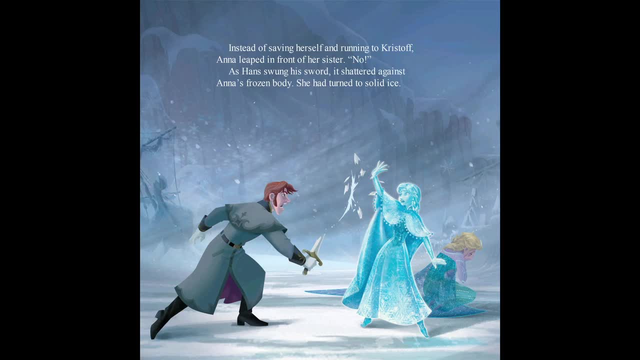 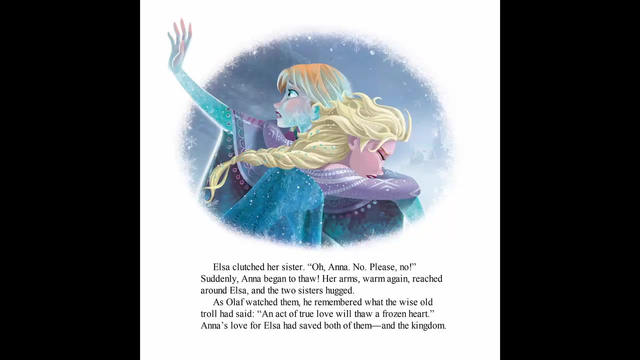 No. As Hans swung his sword, it shattered against Anna's frozen body. She had turned to solid ice. Elsa clutched her sister. Anna- No, Please, no. Suddenly Anna began to thaw. Her arms, warm, again reached around Elsa and the two sisters hugged. 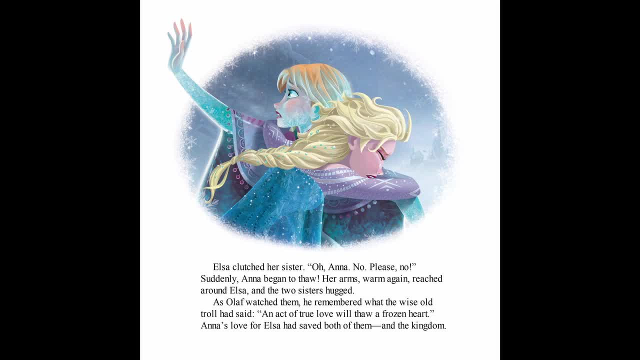 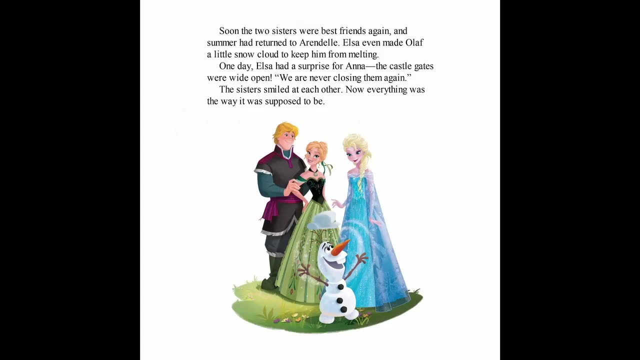 As Olaf watched them, he remembered what the wise old troll had said: An act of true love will thaw a frozen heart. Anna's love for Elsa had saved both of them and the kingdom. Soon the two sisters were best friends again, and summer had returned to Arendelle. 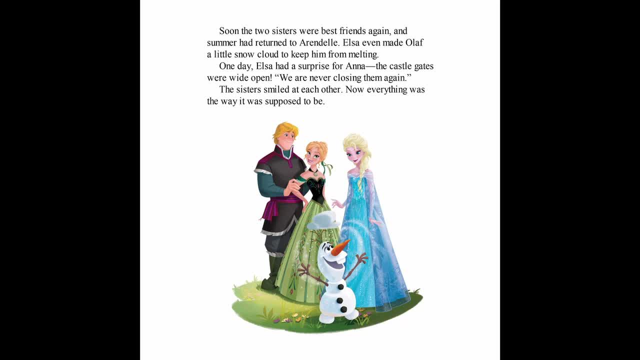 Elsa even made Olaf a little snow cloud to keep him from melting. One day, Elsa had a surprise for Anna. The castle gates were wide open. We are never closing them again. The sisters smiled at each other. Now everything was the way it was supposed to be.